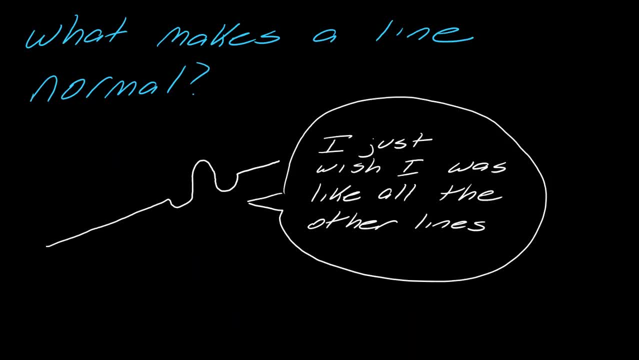 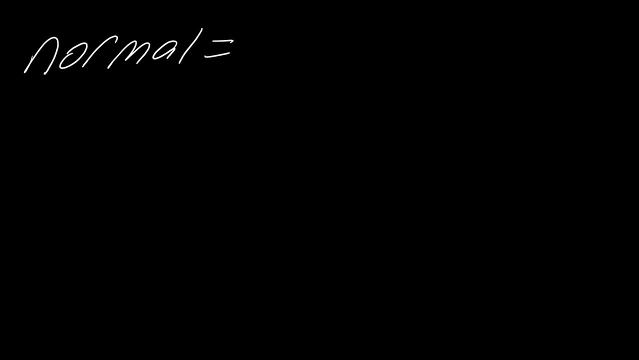 so make sure you check that out. So let's talk about what makes a line normal. So it's very, very simple actually. So a normal line is just another word for a perpendicular line And, by the way, another word for normal or perpendicular is the term orthogonal. 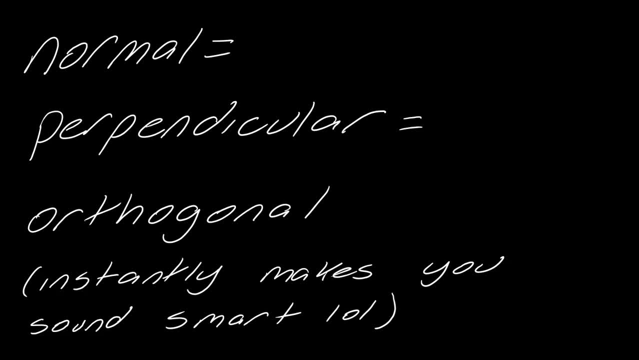 I love the word orthogonal. I think it makes you sound instantly smart, So you can say that you know, oh, you know, this line is orthogonal to the other. So practice it, have fun with your friends. So where do we actually encounter normal lines? Why would we care? So one application of 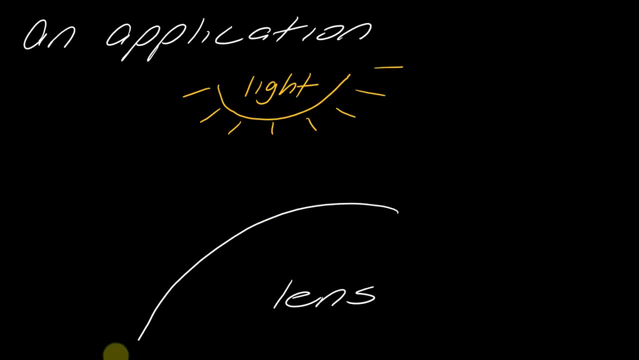 this actually has to do with lenses. So if you think about how a lens works, so it's usually like a you know a lens is a lens. So it's usually like a you know a lens is a lens, So it's a curve, like think about like any, any lens that you want, So it's usually got a curve. 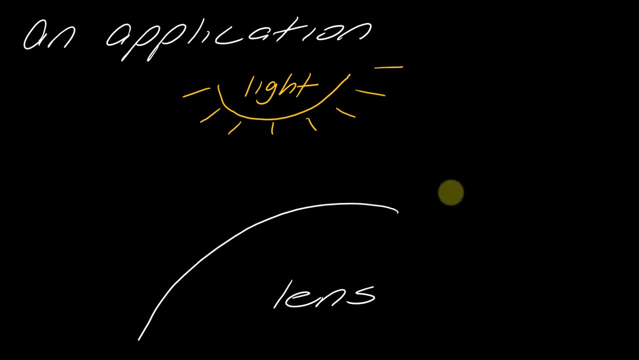 on it And usually when we have kind of these circular type curves, a lot of times these will be equations that are in terms of X and Y. So these are the types of equations that we usually want to have an implicit differentiation, or we might have to implicitly differentiate. 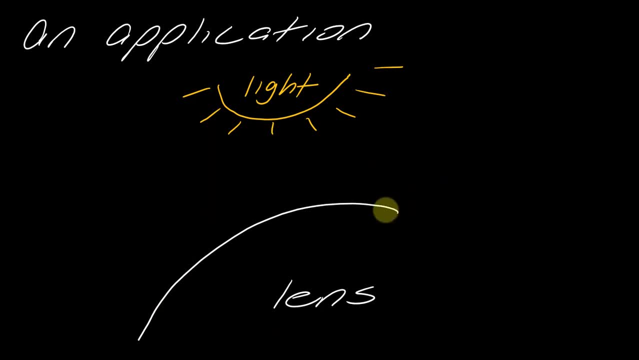 So I've got this lens, again, pretend the equation for it's in terms of X and Y, and then I've got a light coming into the lens, So the light will enter the lens like this, And so this is our curve, that we would have this X and 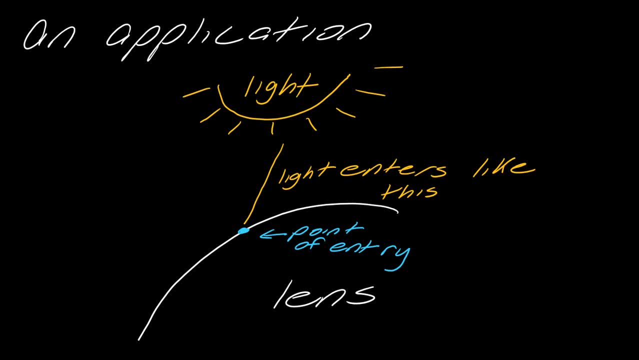 Y equation for: And let's say that this is the point of entry, right here. So at this point of entry we can come up with this tangent line. So it's tangent to the curve at this point. And so now, this is where the normal line comes in. So remember what the word normal means. 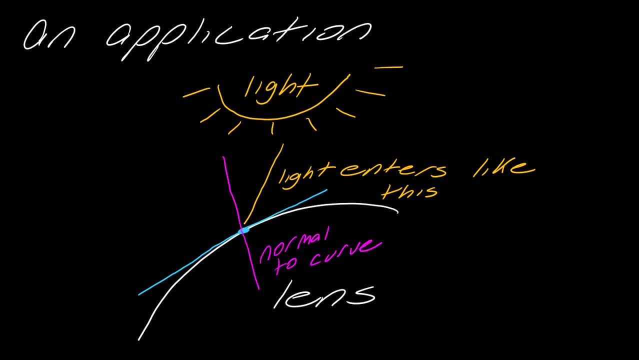 So it here's the normal to the curve. So it's going to be the line that goes, that is perpendicular to that tangent line, And so what this actually does, this actually is what will determine how the light bends. So when you know, kind of, how these two lines meet, you can figure out how the light is. 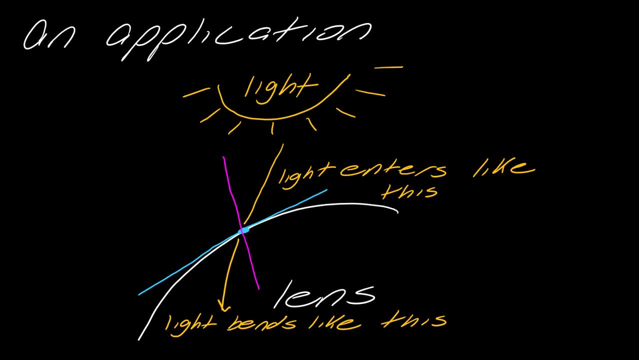 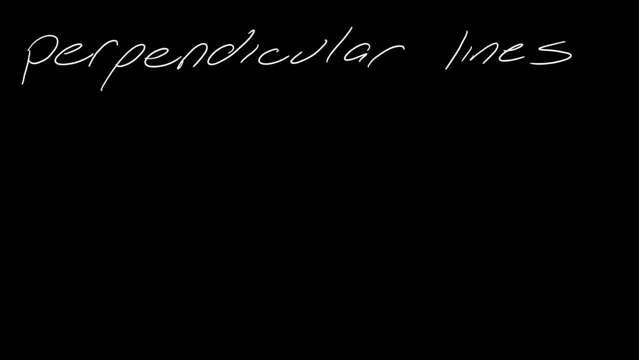 going to, to bend basically, And this is a process, by the way, known as refraction. So that's just a really quick explanation of why would you ever want to come up with this? So, just talking about refraction with lenses, that's one popular application. Okay, Now let's talk about 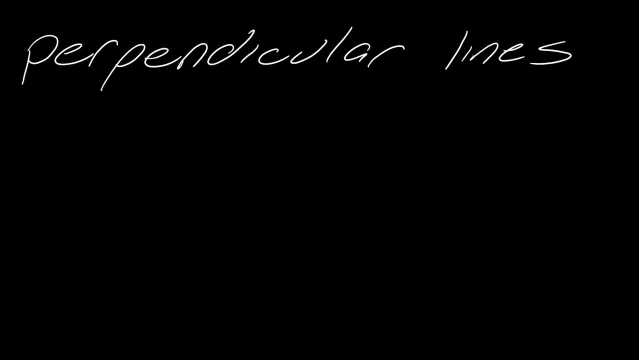 perpendicular lines. for a second, What makes two lines perpendicular? So perpendicular lines have negative or opposite reciprocal slopes. So if you forgot what that means, so let's pretend I have the slope M equals one third. then the opposite reciprocal slope would be: M equals positive three. 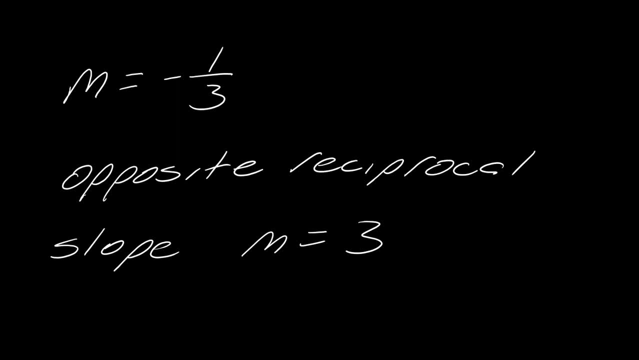 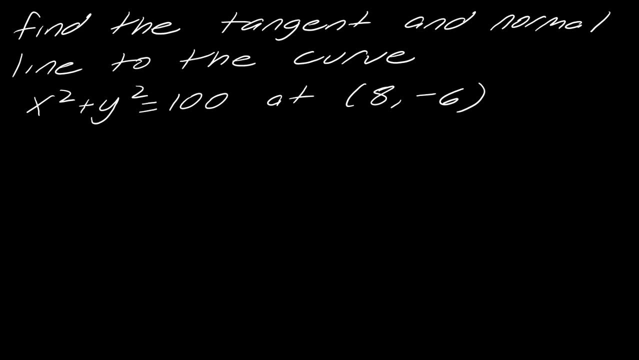 So notice, it's both a reciprocal and it has the opposite sign. So that's what I mean by opposite. Okay, So, given that little quick explanation, now what I want to do is I just want to kind of walk you through. how do you actually find these things? So I've got this nice simple equation here. So X squared plus. 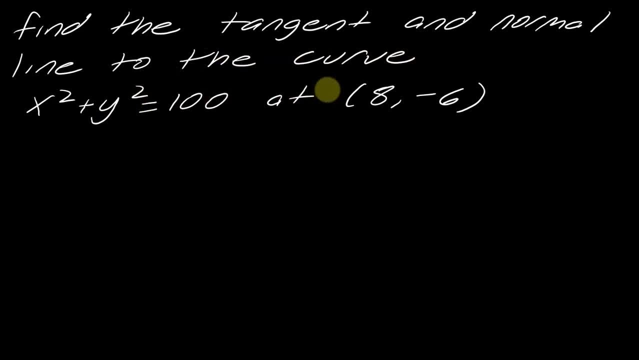 Y squared equals a hundred. So I want to find the tangent and the normal line to this curve. So these are two totally different processes. In general, you're going to want to start with the tangent line first. So the word tangent usually means take a derivative. It actually always means take a. 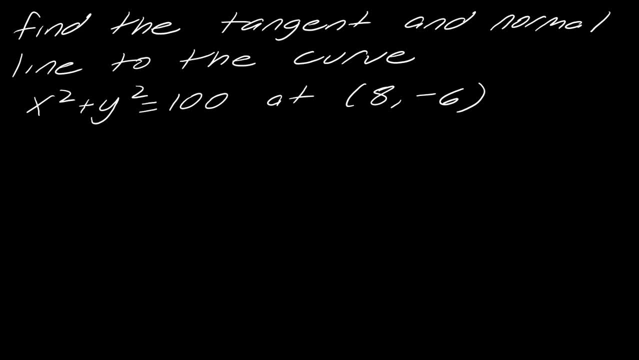 derivative. So we're going to take the derivative of this. So you should already know how to implicitly differentiate. If you don't know how to implicitly differentiate, you should already know how to do it. If you don't, make sure you go back and watch a video about that. So if I implicitly 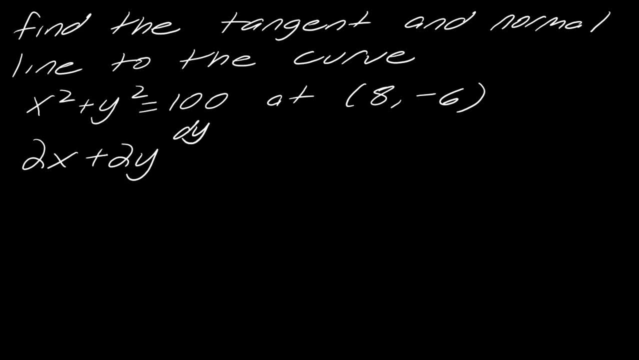 differentiate, I get two X plus two Y. dy dx equals zero. And so if I solve for dy dx, so I get: dy dx equals negative two X over two Y, So this is just: dy dx equals negative X over Y. Okay, So remember what these formulas stand for. 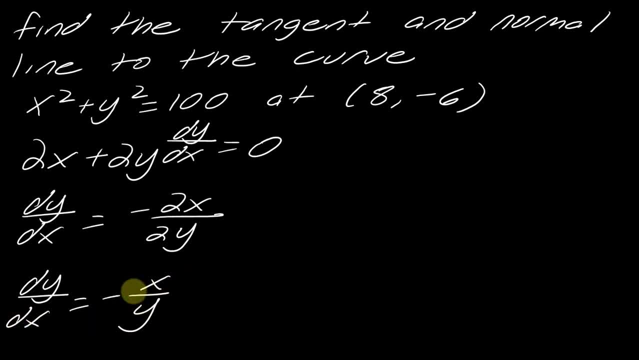 This is not the tangent line, right? This is how you figure out what the slope of a tangent line would be. So this point, you know, this point is on the curve, right? So if you, if you plug this in, you'll get 64 plus 36, that does indeed equal 100, right? So the point that you get here has to. 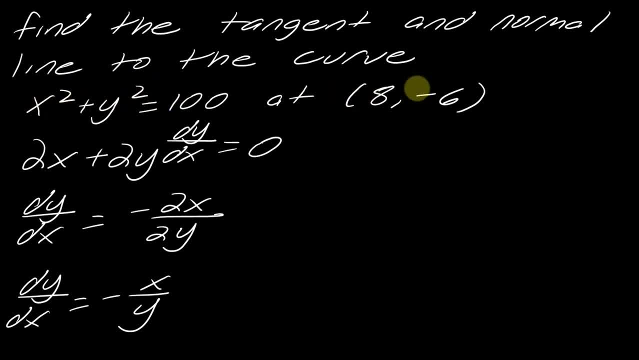 be one that's actually on your, your curve, And then, after you find that point, you plug that point into your slope formula. So we're trying to figure out the tangent line. So I have a point I need, I need the slope. So 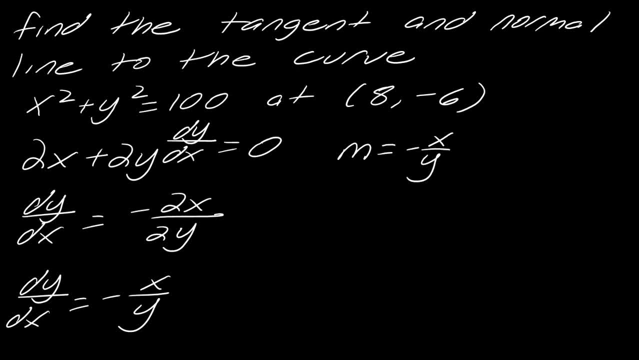 my M in this case is going to be: so I take negative X over Y and I just plug in this coordinate, So this becomes negative eight over negative six. So this really comes out to, let's see, was it four over three. So there's my, my slope, That's my M. Okay, So now I'm just